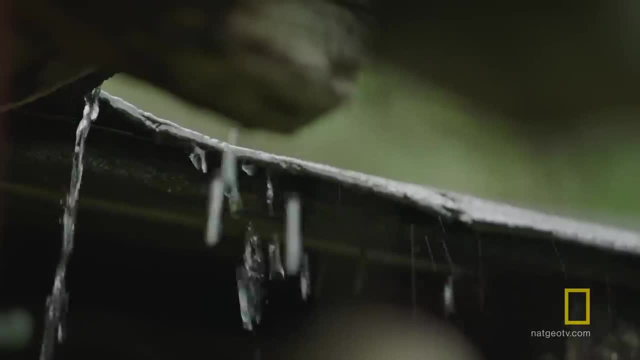 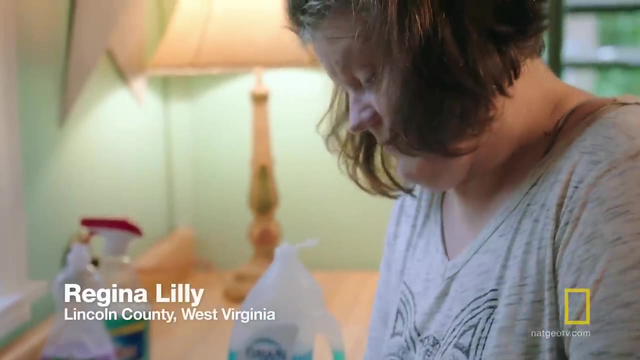 sludge that's leaking into the drinking water. Everybody's will is pretty much is contaminated in one form or another. So I don't use the water to cook. I use it to do the dishes, But that's about it, because you can wipe the water off. 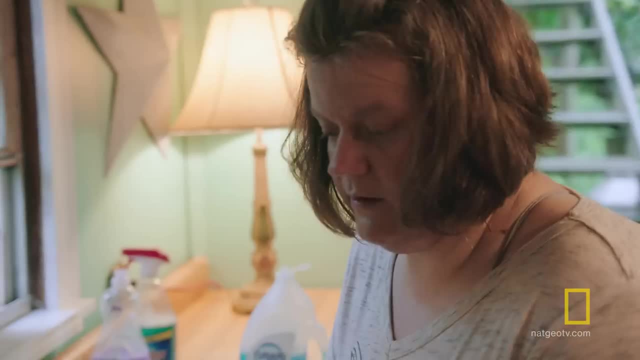 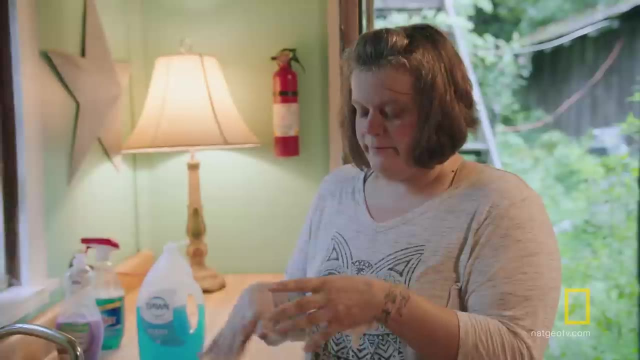 There's a guy that we tend to help out. every now and again He is blind from the water. He could take his water, Turn his water on, put it in a clear water bottle, put his hand over it, sit it for a few seconds. 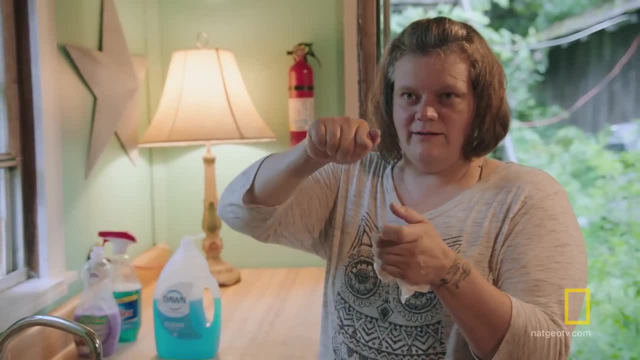 even put a cap on it. take the cap off and take a lighter and light it and water will burn. So yeah, water in here is pretty bad. 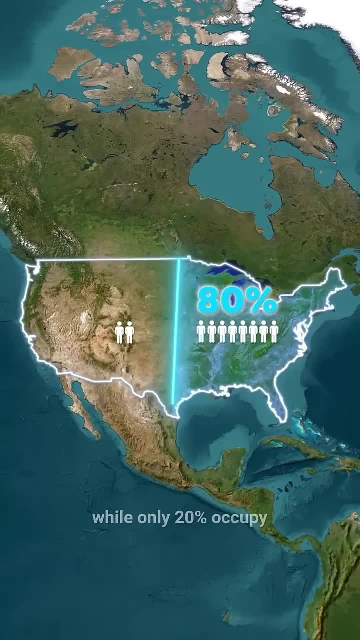 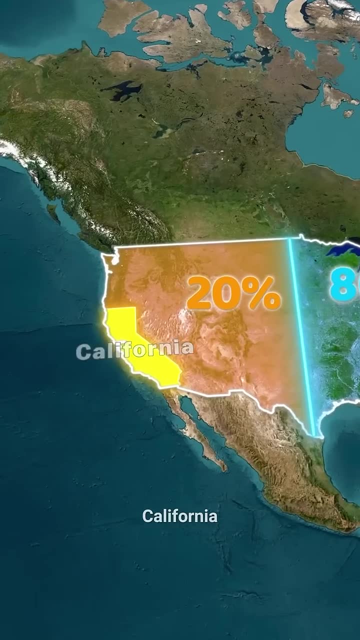 Why do 80% of all Americans live east of this line, while only 20% occupy the western part of the United States? Even more, the majority in the West live in California, Oregon and Washington, within this line, accounting for 11% of all those living in the West. Thus, 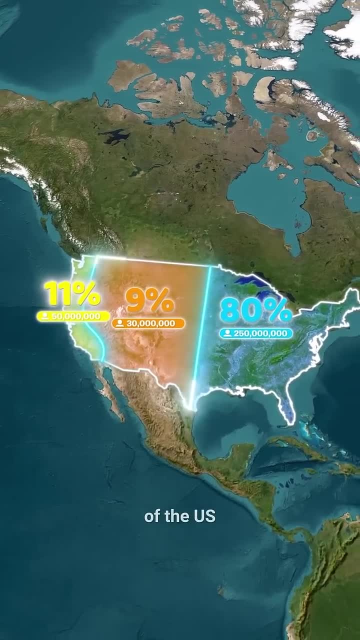 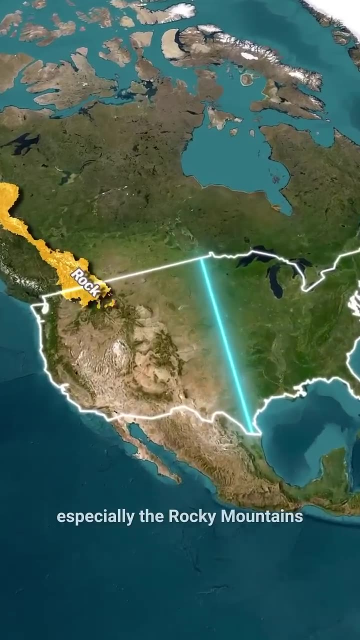 only 9% of Americans live in half of the mainland of the US, which is equivalent to the population of New York City alone. Why is that? The main reason for this is geography, especially the rocky mountains that stretch across the entire country and act as a natural barrier to the 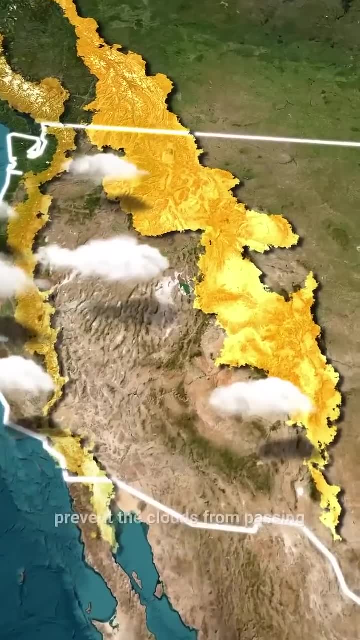 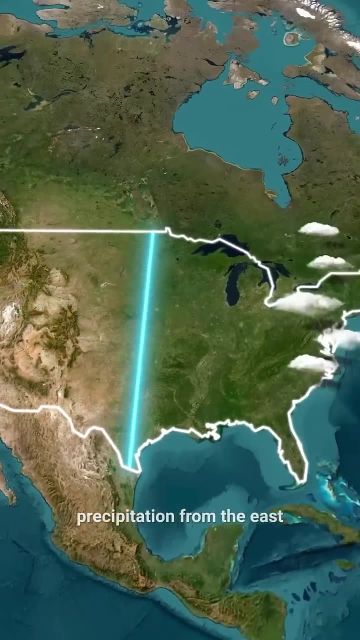 rains coming from the Pacific Ocean. They are so high that they prevent the clouds from passing into the center of the country, and this effect is called rain shadow. At the same time, precipitation from the east can easily penetrate into the depths of the country, but due to winds from the Gulf of 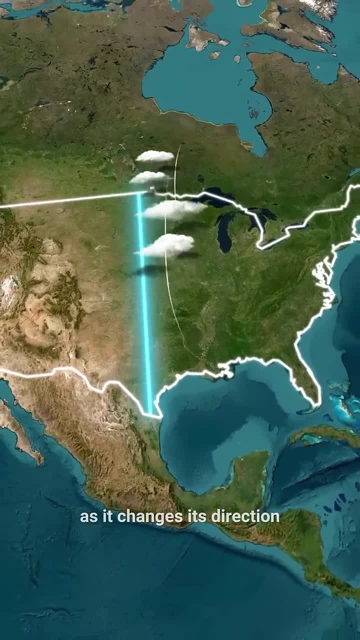 Mexico cannot cross this line as it changes its direction. Because of the lack of precipitation, it creates an area of dry land that is not suitable for agricultural production, and this is the reason why most Americans live in the western part of the US. 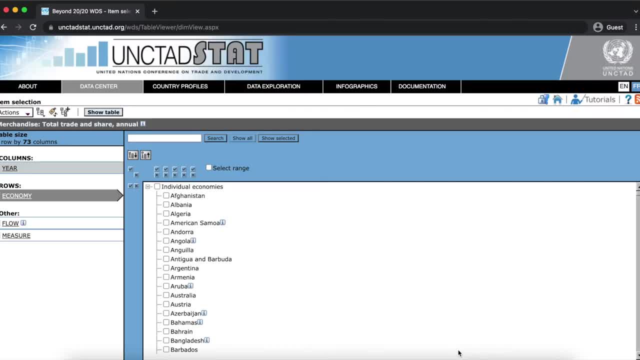 The expand all and collapse all buttons will expand or collapse your view of all the dimension items. So clicking on expand all will open all the groups in that dimension and you'll be able to see each individual item. Clicking on collapse all will put all the items back in their groups.